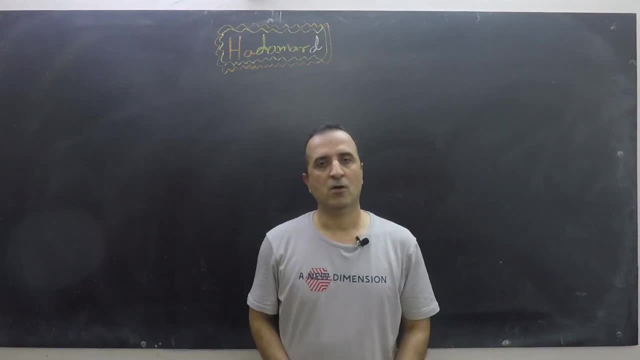 So far we have learned that how to use Hadamard gate on a single qubit. Hadamard gate is a single qubit gate so it can be easily applied to transform a single qubit. However, we can extend Hadamard gate for multiple qubits using tensor product. 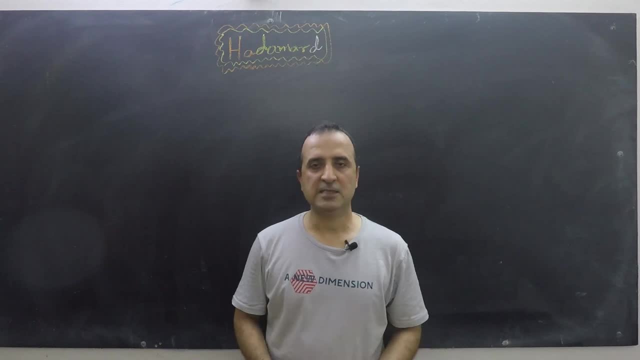 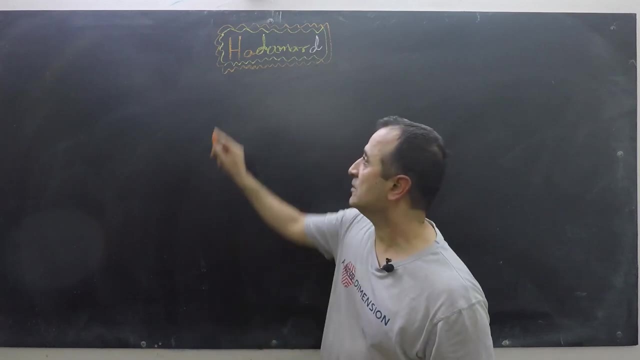 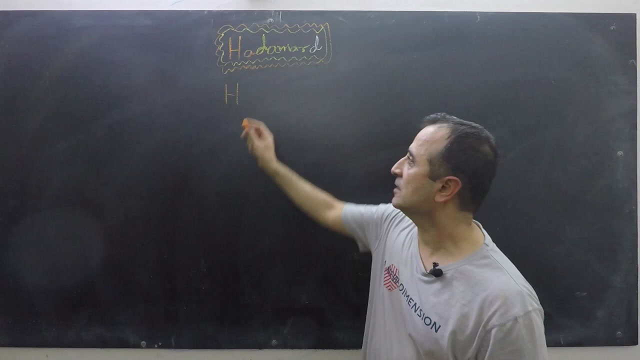 and can apply it on multiple qubits. and this is the subject of this video, that we will learn how to apply Hadamard gate on multiple qubits. So let's say we have given Hadamard gate and we have to apply the Hadamard gate on a two qubit register. In that case, a Hadamard gate will 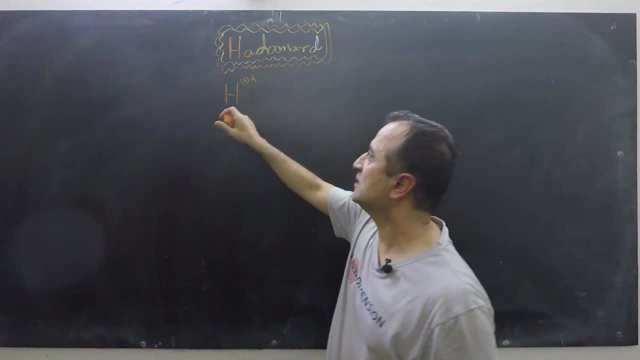 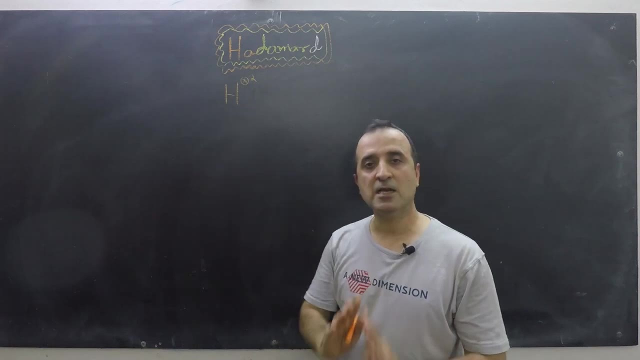 be written as Hadamard gate, tensor product 2.. This tensor product 2 implies that we have to extend Hadamard gate on two qubits. This Hadamard gate is not a single qubit gate, but it's a two qubit gate. 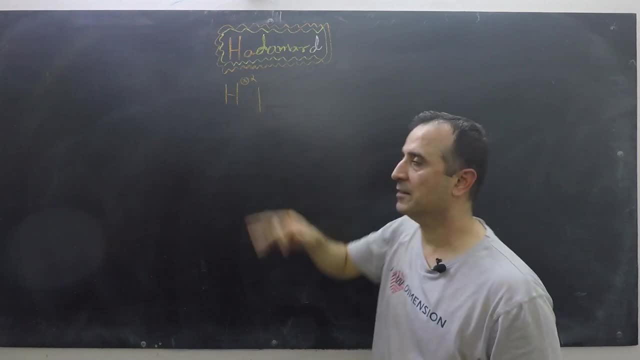 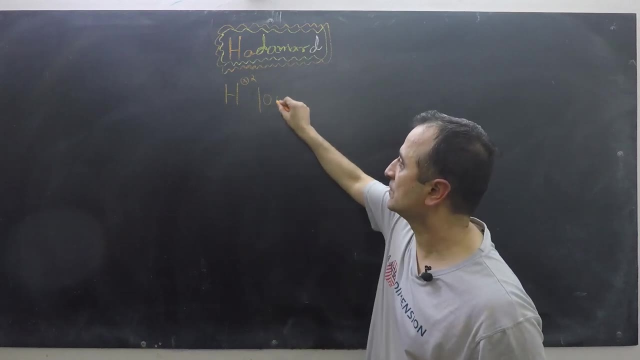 and afterwards we will have a register here which will be a two qubit register For the sake of example. let's say our register contains cat 00. So we have to basically find out what is the outcome of this expression. So there are two. 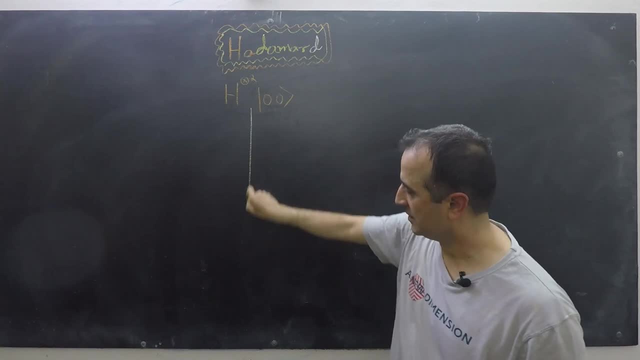 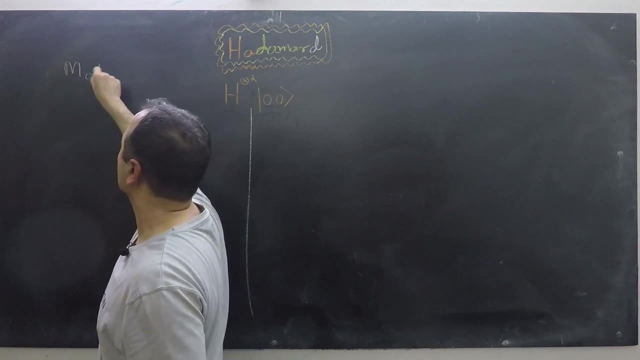 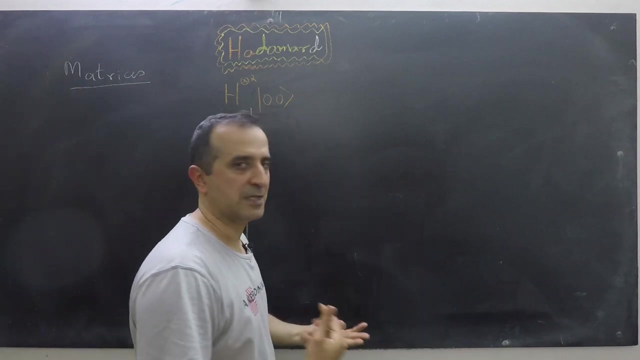 methods to solve this expression. One method is using matrix. So one method is using matrices. The second method is by using the single qubit Hadamard gate. So second method is using the fact that Hadamard gate, on cat 0, is a single qubit. 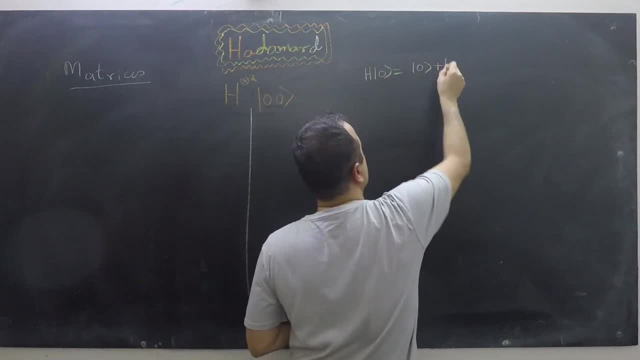 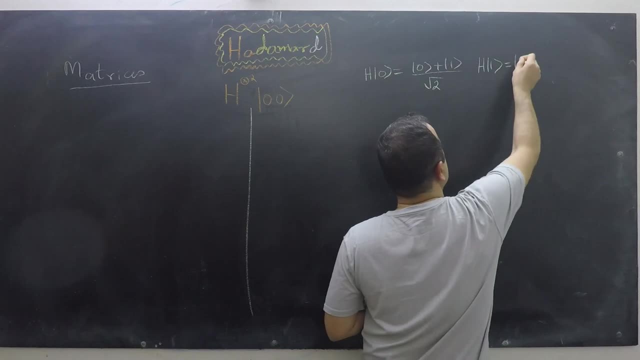 Hadamard gate on cat 1 is equal to cat 0 plus cat 1 divided by a square root of 2.. And Hadamard gate on cat 1 is equal to cat 0 minus cat 1 divided by a square root of 2.. 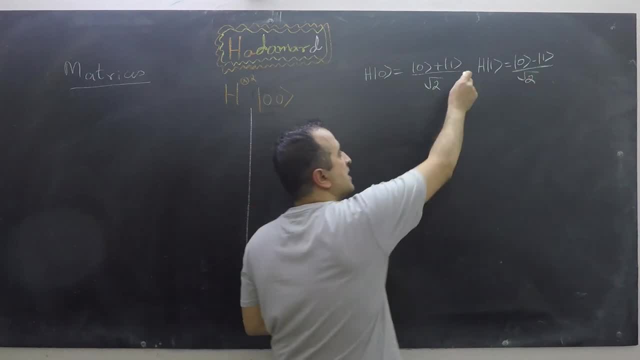 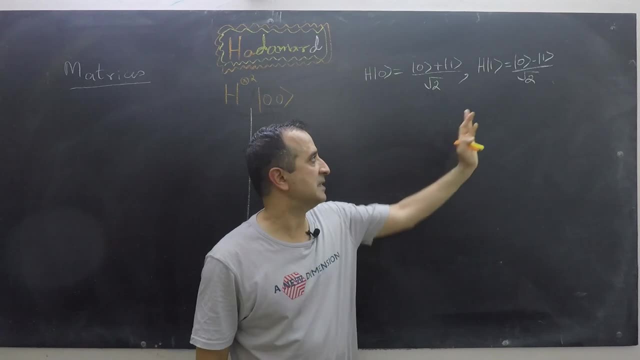 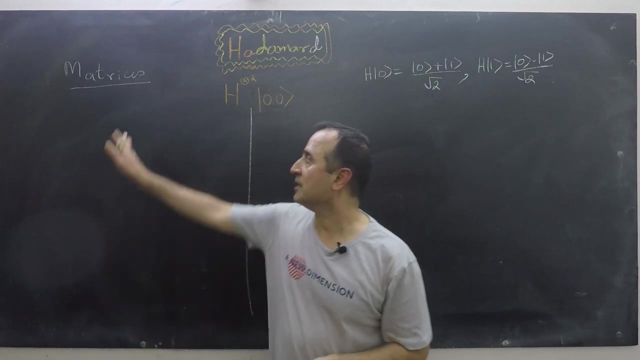 The second method employs this concept, whereas the first method uses matrices. In practice, we use this method more often because it takes much less time and this method works when we have to use Hadamard gate on more than two qubits. But this method is good to understand the basic concept and to develop intuition. 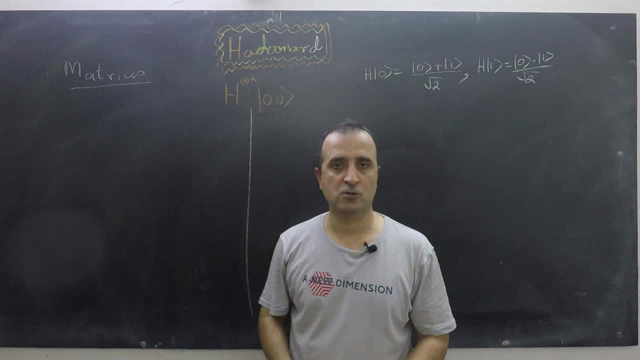 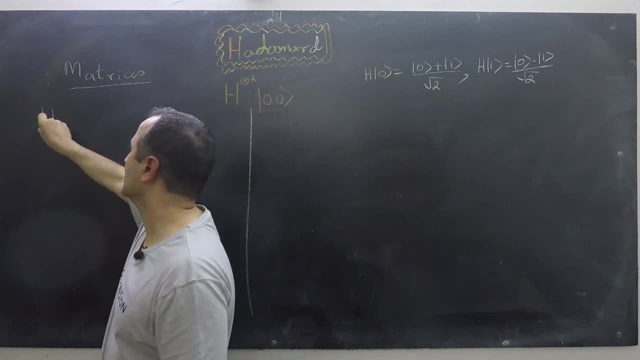 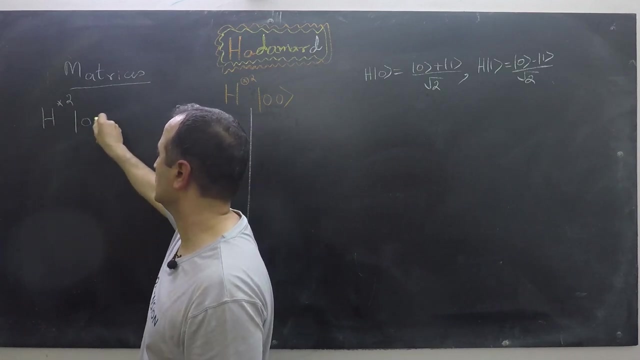 So let's start with the matrices method, which is not commonly used. but it is good to develop intuition. So what we are given is that we have to apply Hadamard gate tensor product 2 on a two qubit register which has cat 00 in it. So this implies that I have to tensor put Hadamard gate. 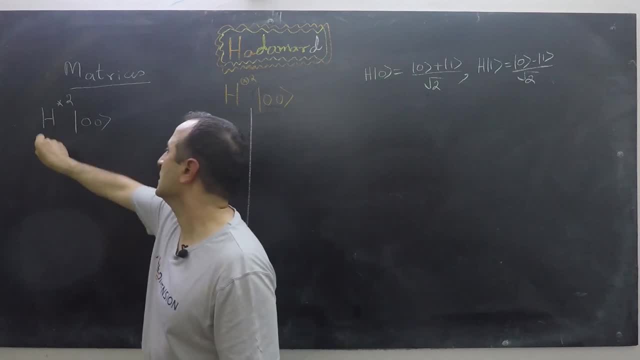 with itself. So this implies that I have to tensor put Hadamard gate with itself. So this implies that I have to tensor put Hadamard gate with itself. So this expression implies, This expression implies That I have to do this operation: Hadamard gate tensor project with Hadamard gate. 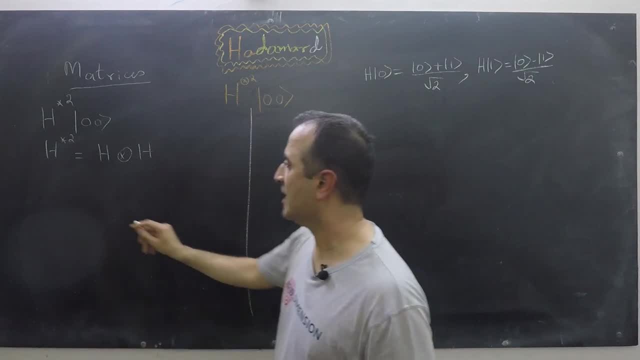 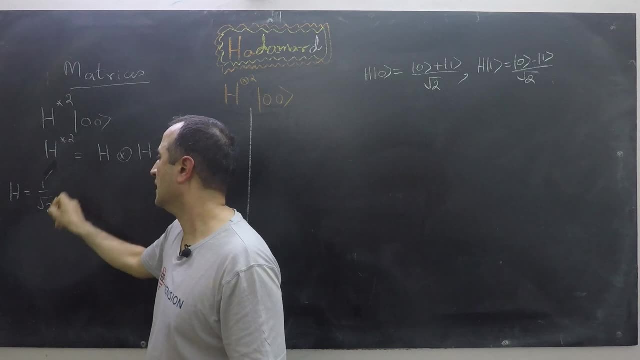 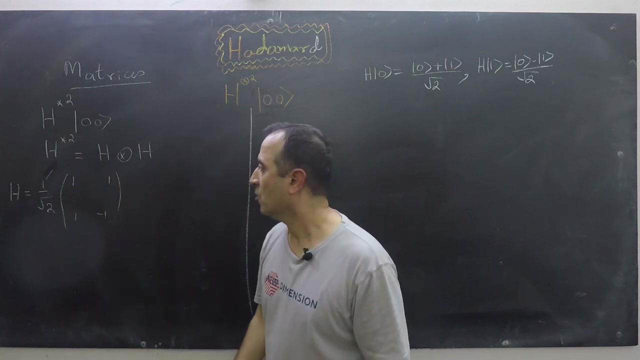 So we know what is Hadamard gate is. So we know Hadamard gate in the matrix form is that we have 1 over square root of 2, and then we have 1, 1, 1 minus 1. so now what will be Hadamard gate? tensor product for electronic resource. 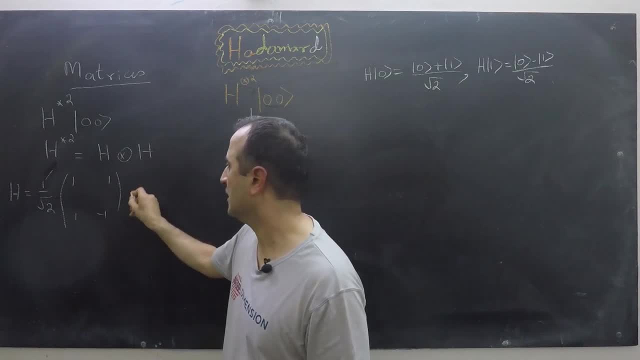 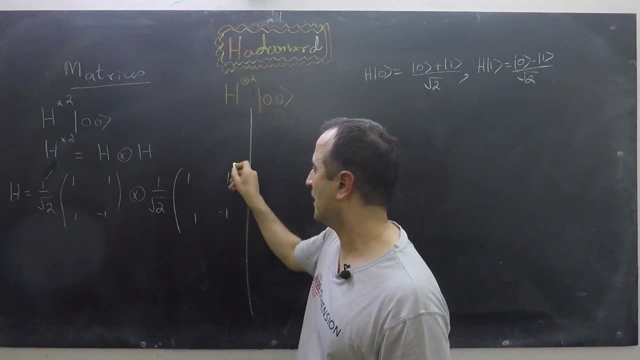 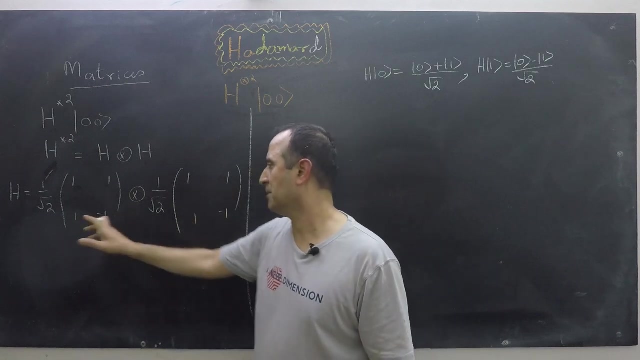 itself. So when we say tensor, product with itself, then it implies that this number multiplied by this whole matrix, this number multiplied by this whole matrix, this number multiplied by this whole matrix, and this number multiplied by this whole matrix, So what we will get 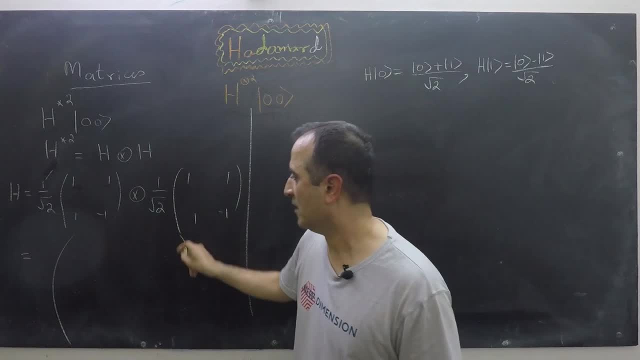 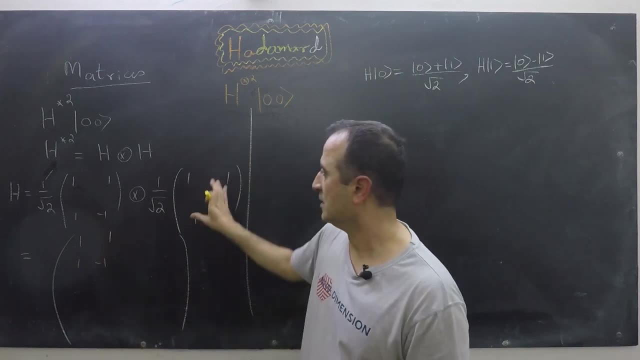 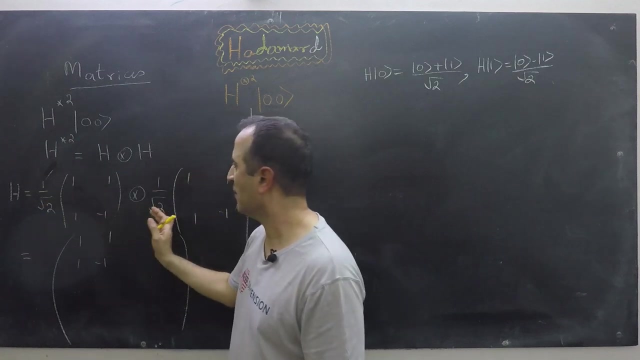 at the end is that when we multiply 1 with this whole matrix, we will have here 1, 1, 1, minus 1.. So this here is this whole matrix, and these normalization constraints will also multiply with each other, So we will have here 1 over 2.. So this I'm just writing. 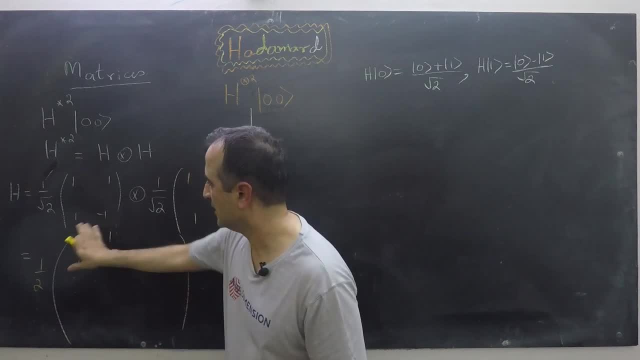 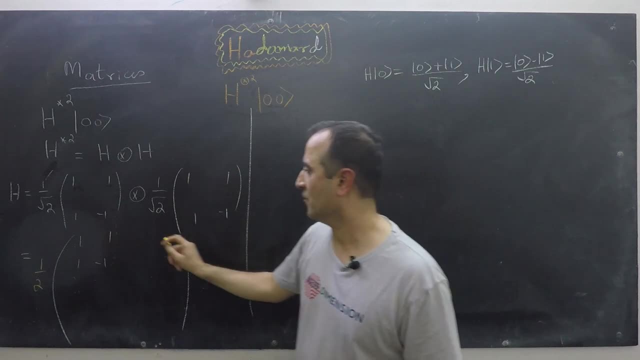 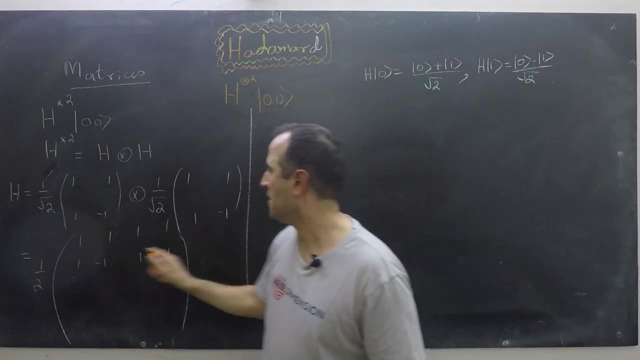 here dots for the sake of understanding that this is this whole matrix multiplied by 1, similarly, 1 multiplied by this whole matrix, we will have here 1, 1, 1 minus 1. similarly, this 1 multiplied by this whole matrix, we will have here 1, 1, 1 minus 1. and finally, we have minus. 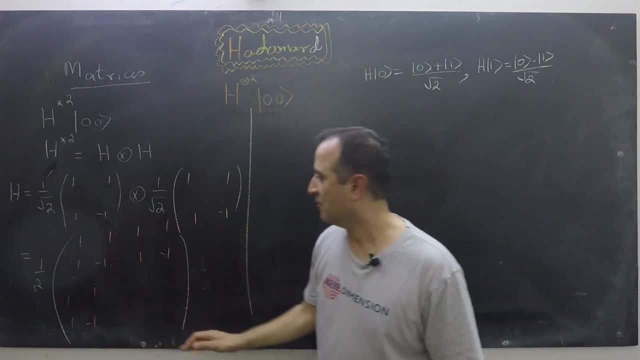 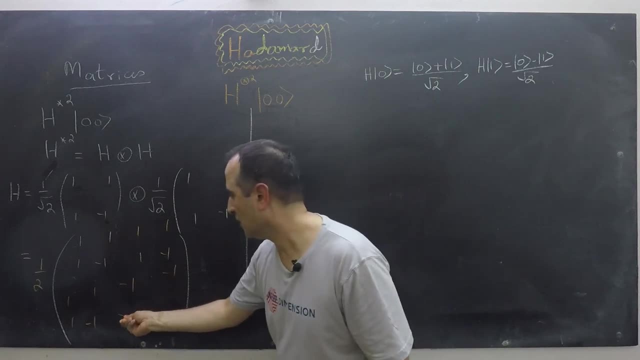 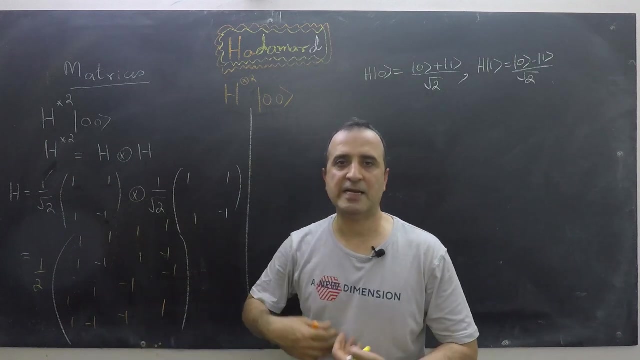 1 multiplied by this whole matrix. so the last entry will have all the sign reversed. so you have here minus 1 minus 1, minus 1, and this minus 1 will become plus 1. so that's our hadamard, this, this is our hadamard gate tensored with itself. this is our, this expression. similarly, we can do: 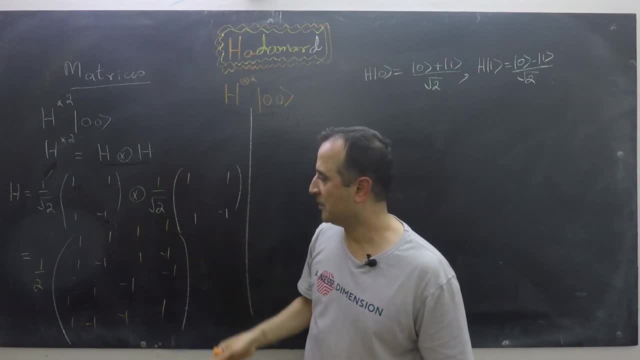 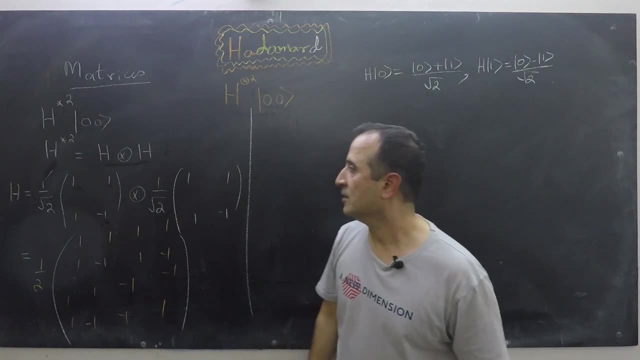 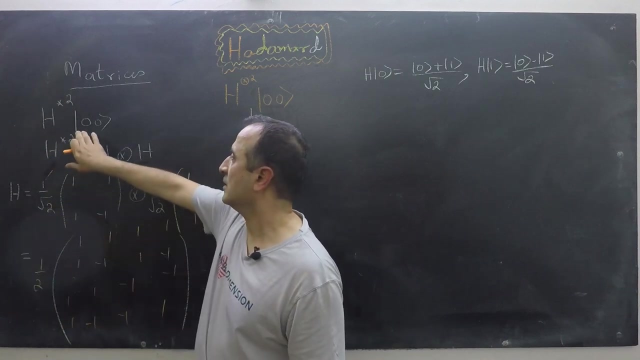 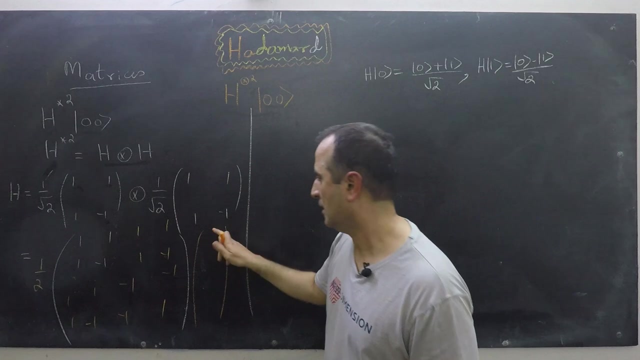 hadamard gate tensored three times, we have to basically once again tensored this matrix with another hadamard gate, but that's, we are not doing this video. so now i have to find result of this thing. so i have found where this is, which is this. now i get 0. 0 is a 4. is a 4 elements vector, the 4 dimensional vector whose 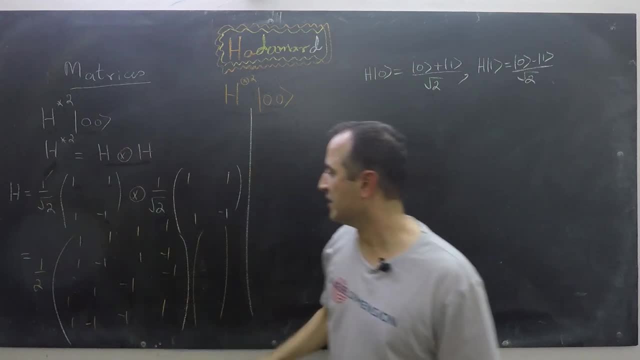 first entry has 1 and rest of the entries has 0 in it. so we will have here 1 0 0, 0. now we multiply this matrix with this vector and we will have our final result. so in this case, our final result will: 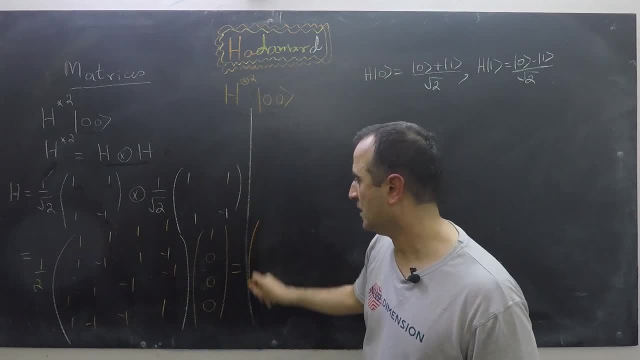 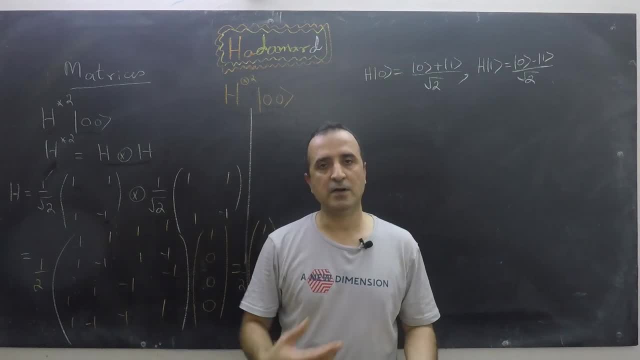 matrices method. but matrices method becomes very difficult when we have more than 2 qubits register. we have 10 qubit register. very difficult to write a huge matrix for 10 qubit register. so we usually use and this method. so now let's start with the second method. so our second method is extremely simple. so in our second 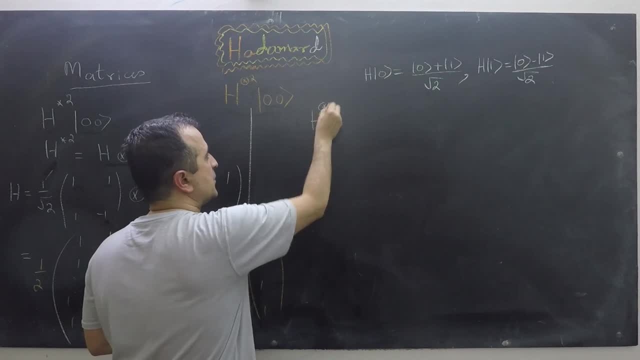 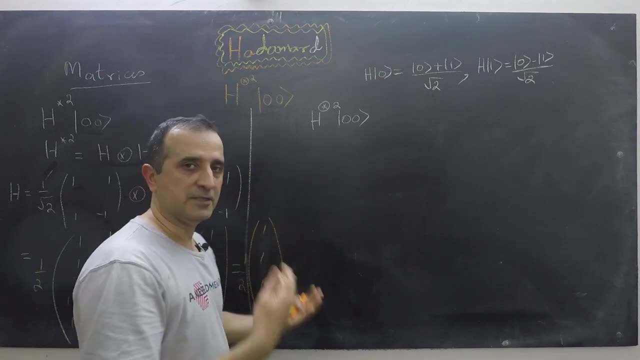 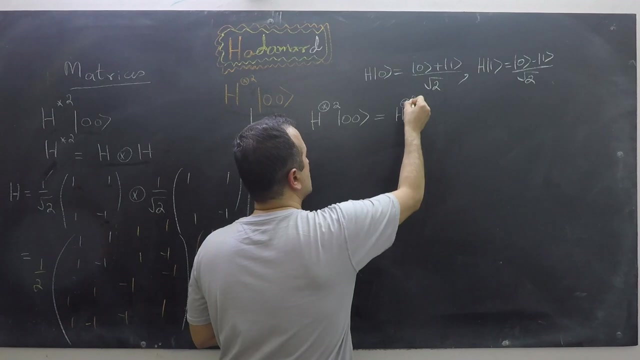 method we have to calculate a hadamard gate tensor, product 2 with cat 0, 0. so first of all we can write this cat 0, 0 as cat 0 times cat 0. so we can write it like this: hadamard gate, tensor, product 2 and we: 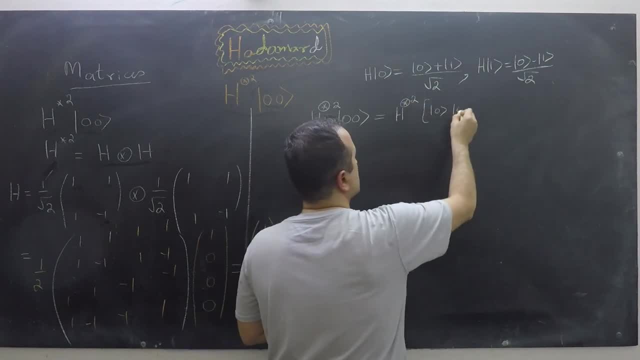 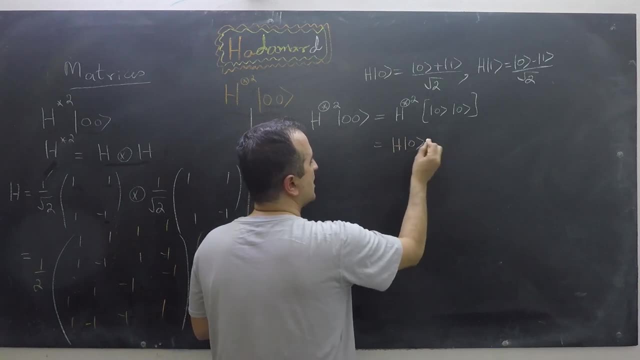 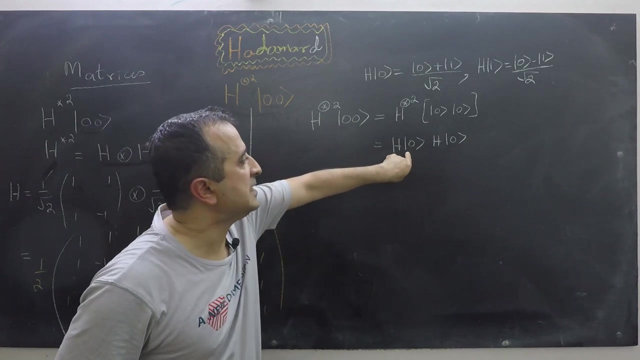 can write here maybe cat 0 times cat 0, and then we can basically simplify it like this: cat, hadamard gate 2, cat 0 and had amad gate to catch you. so this is our second method we just have. we are applying hadamard gate on each individual.